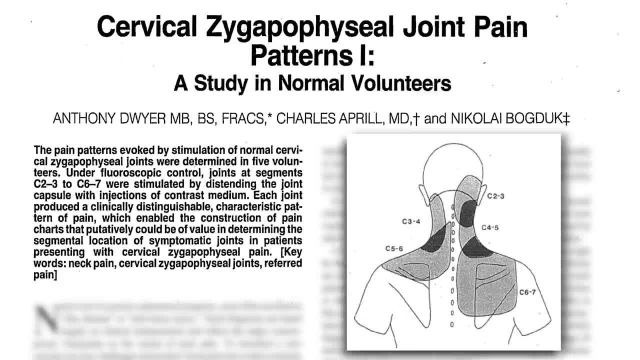 the discs such as Slipman et al in 2005.. And Dwyer et al in 1976, is well known for stimulating the zygopophysial joints in asymptomatic subjects and mapping their reported pain. The last consideration, and kind of the focal point of this video, relates to 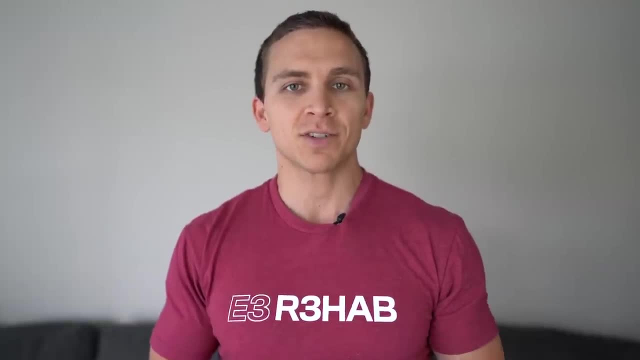 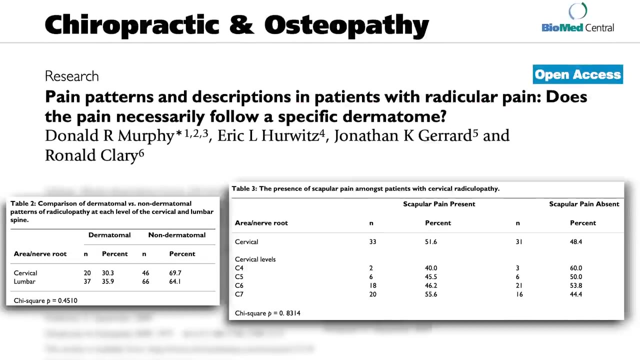 irritation of the lower cervical nerves. Now you might generally associate this irritation with neck pain and this pain down the arm in a nice dermatomal distribution, but Murphy et al in 2009 found that this occurs in less than two-thirds of cases and around 50% of. 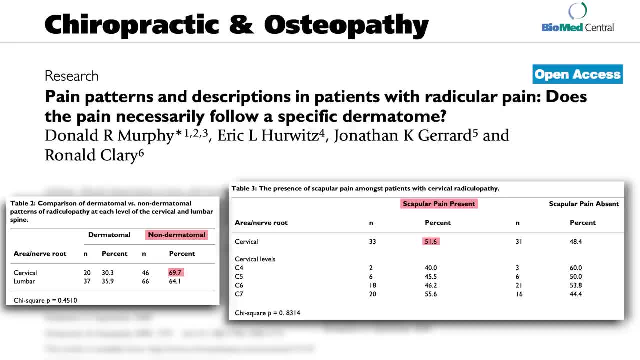 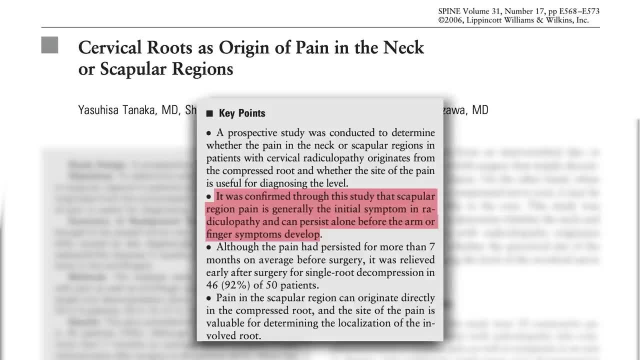 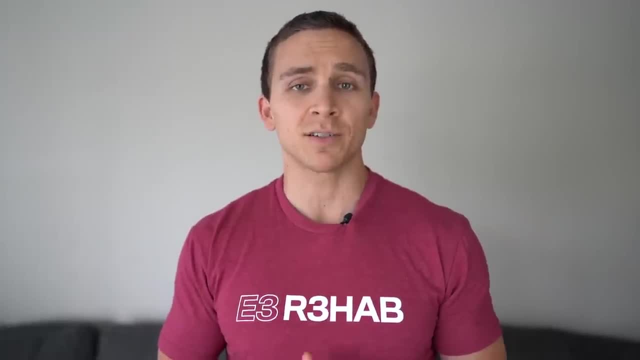 people report pain in that rhomboid area. In fact, Tanaka et al in 2006 reported scapular region pain is generally the initial symptom in radiculopathy and can persist alone before the arm or finger symptoms develop, And in some cases it might be the only symptom that ever really occurs. So, although you 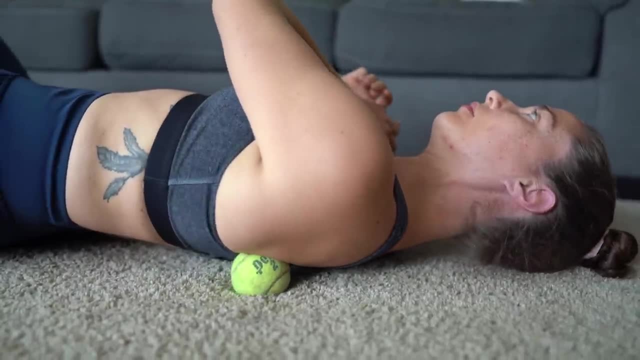 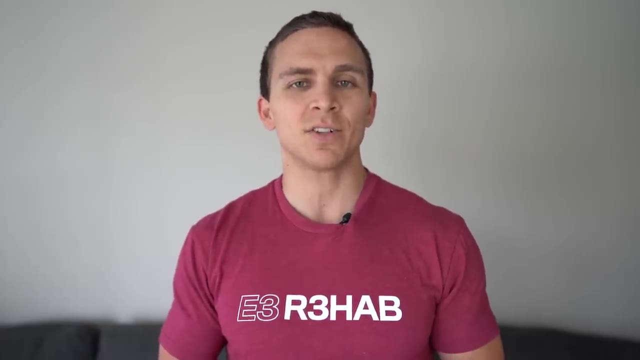 might be experiencing discomfort in the rhomboids. that sensation is likely more of a secondary response. Also, I understand that issues with the neck or a nerve sounds scary to a lot of individuals, but it doesn't mean that anything is damaged, pinched etc. I just like to think of it as 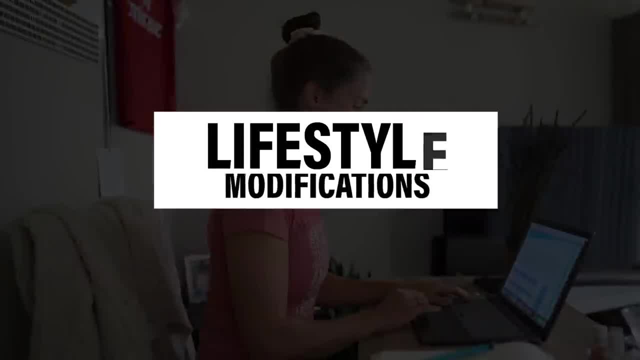 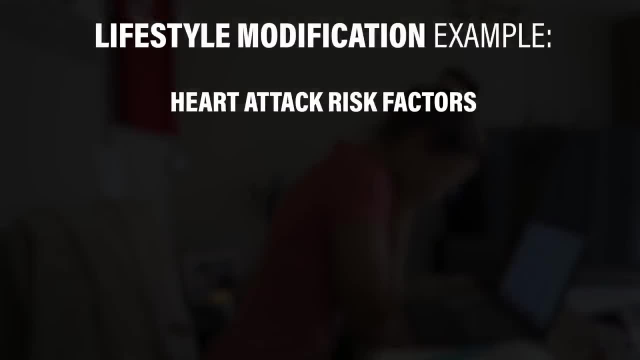 certain tissues being sensitive Lifestyle Modifications. A key tenet in rehabilitation is to modify the modifiable contributing factors. For example, if you are worried about experiencing a heart attack, your age and family history are non-modifiable risk factors. You can't change those. However, you can change your smoking, dietary or exercise. 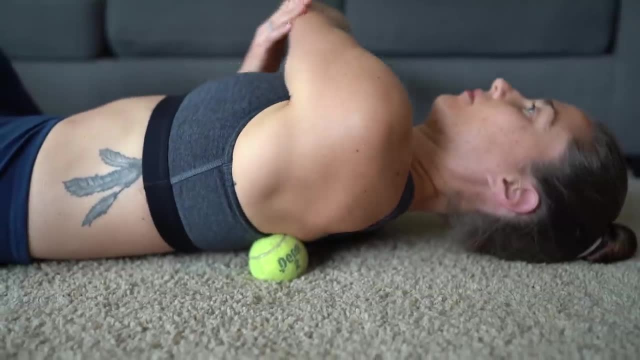 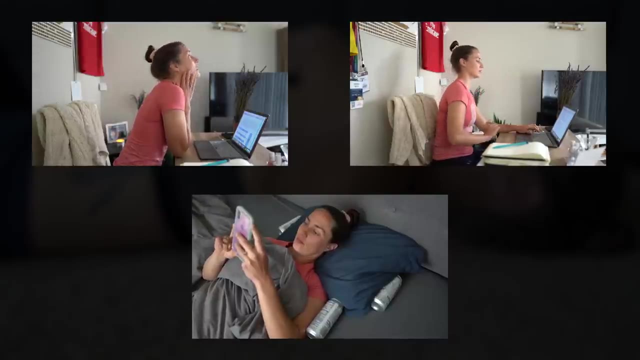 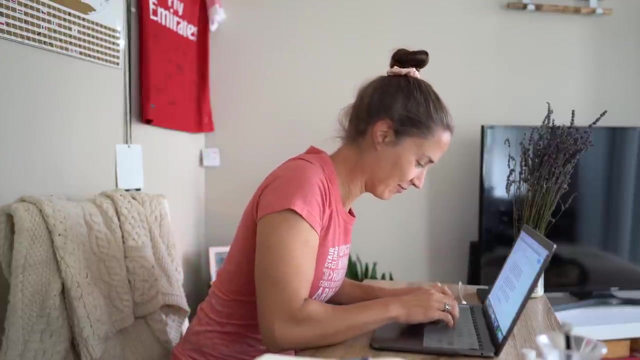 habits. Those are modifiable. In the case of the scapular pain, three aspects of your life worth examining are stress, sleep and prolonged inactivity, as they might be contributing factors. However, I also understand that sometimes these things aren't really modifiable, secondary to unique circumstances. 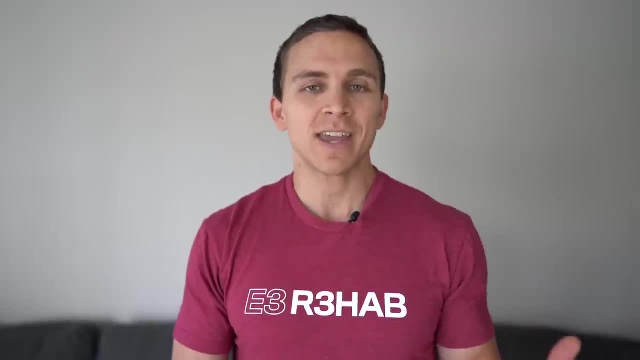 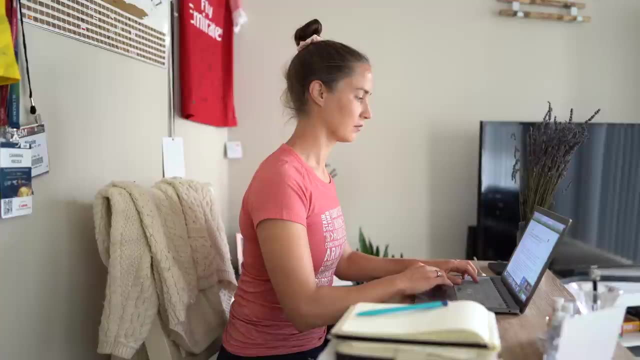 like a newborn child or a dad, a deadline at work. Change what you can, don't worry about what you can't- And I know these things aren't sexy quick fixes, but they're really important For prolonged inactivity. keep it simple If you know you're going to be stuck at the computer for hours on end. 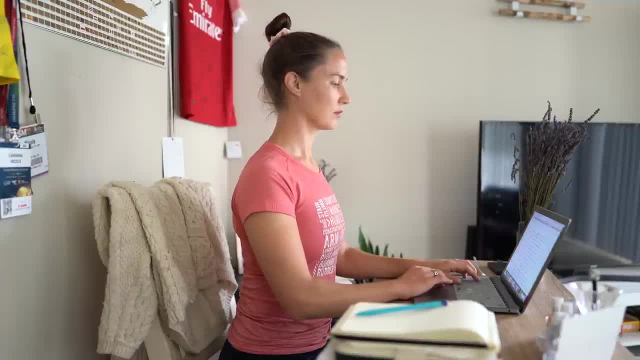 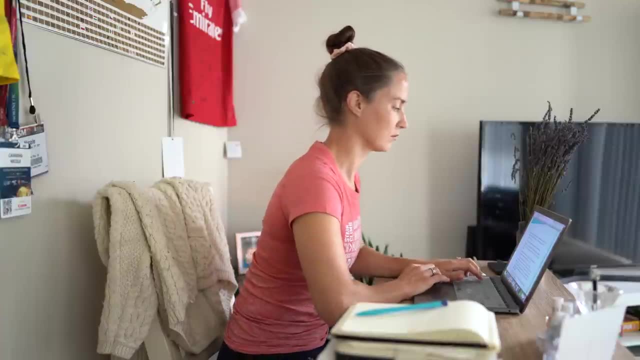 plan some active rest breaks if you're able to like walking or the exercises I'm going to outline. As far as posture goes, don't try to maintain a quote-unquote perfect posture. You might feel better sitting up tall, while someone else feels better slouching. 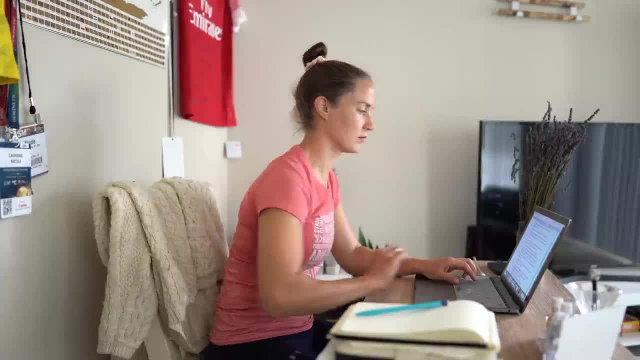 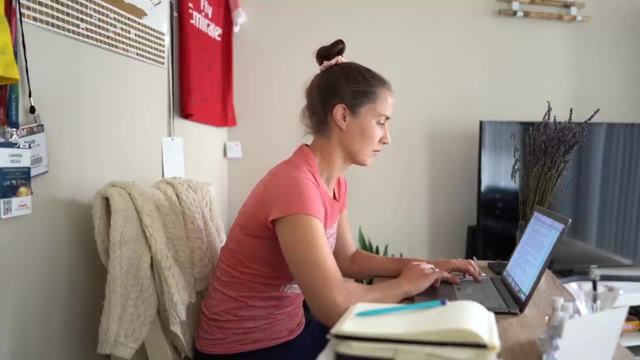 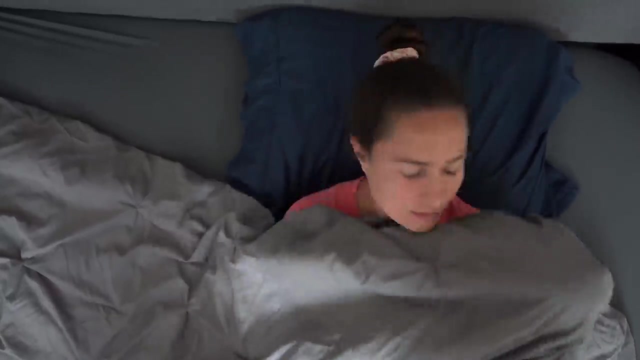 But more than likely you're going to be frequently alternating positions and finding what's comfortable for you. Trying to maintain your shoulders back and down all day can actually exacerbate symptoms. Poor sleep quality and or quantity can magnify symptoms as well, and discomfort can also make it difficult to fall asleep. 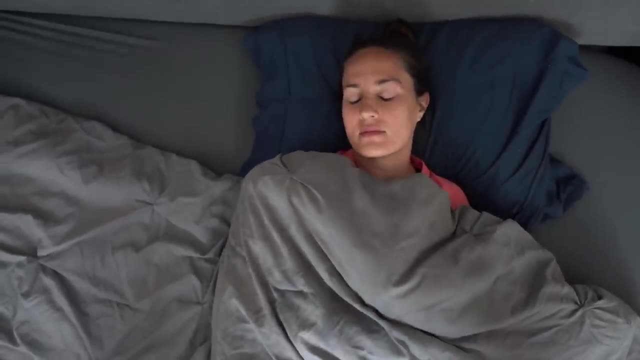 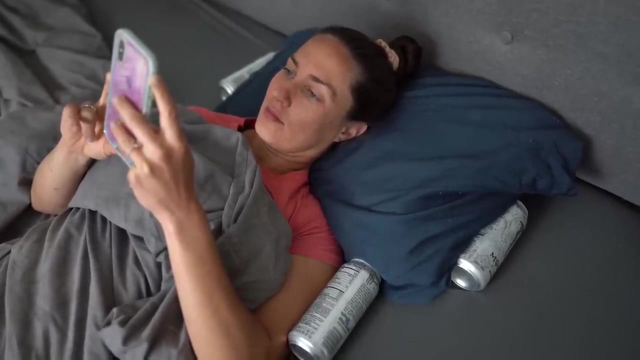 Once again, though: if your sleep is impaired for reasons out of your control, no worries. However, if it's impaired because you're drinking caffeine at night or staring at your phone in bed, those might be things worth changing Now. if you can't get comfortable, this recommendation is similar to posture. 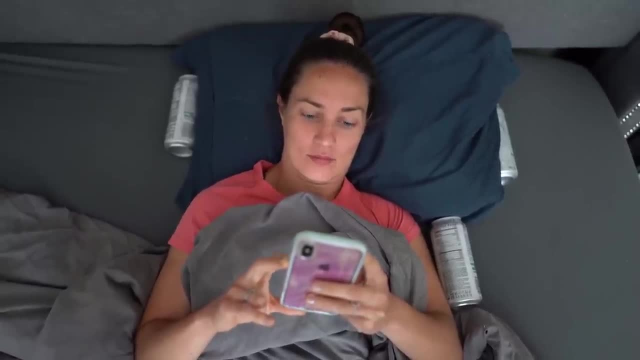 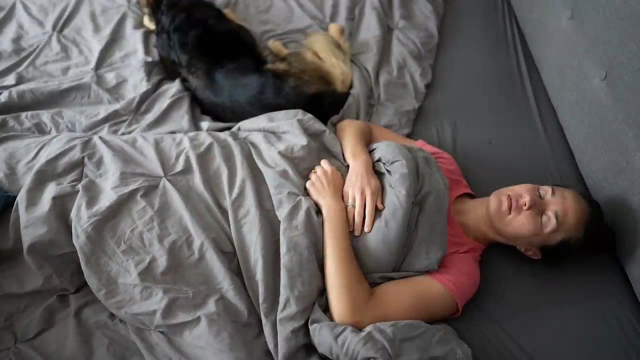 There's not a perfect neck position, so explore options. Line on the affected side, on the unaffected side, one pillow, two pillows flat on your back or head and neck elevated. There are various reasons why different positions can help alleviate symptoms. 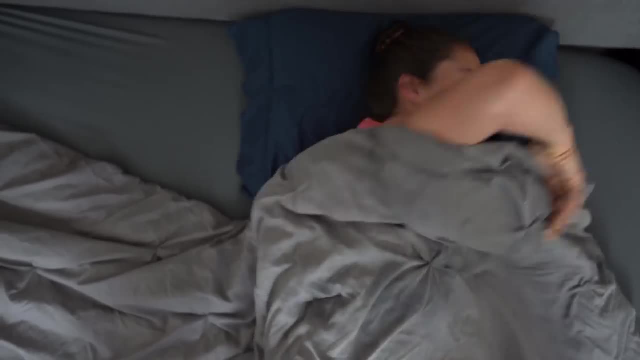 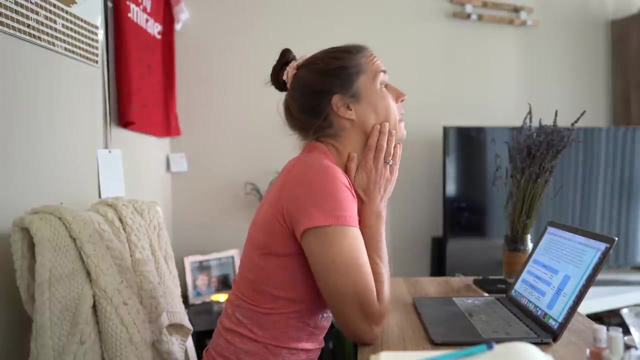 for different individuals, but the most important thing here is making sure you're comfortable. Finally, stress can also increase the sensitivity of nerves, so if you notice your symptoms are triggered by high stress situations, you can try to alter the situation or your reaction to it. But if you can't, 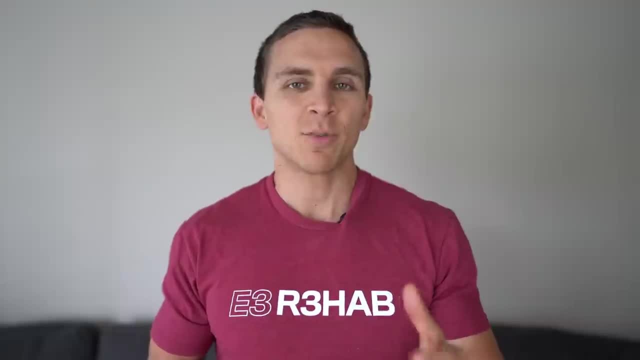 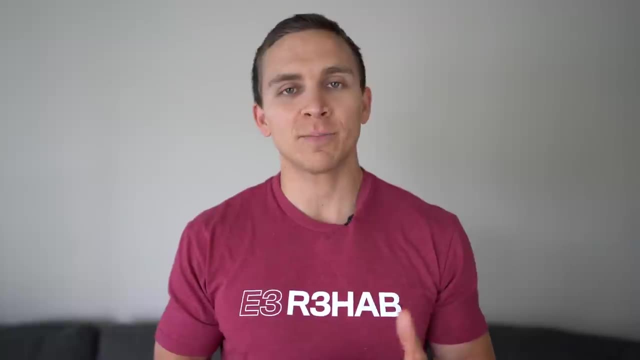 no big deal. Plenty of other things to focus on. I'm going to provide a sample, exercise, progression and parameters, but I need to highlight that the theme here is based on a simple, practical quote by Louie Gifford: start easy, build slowly. 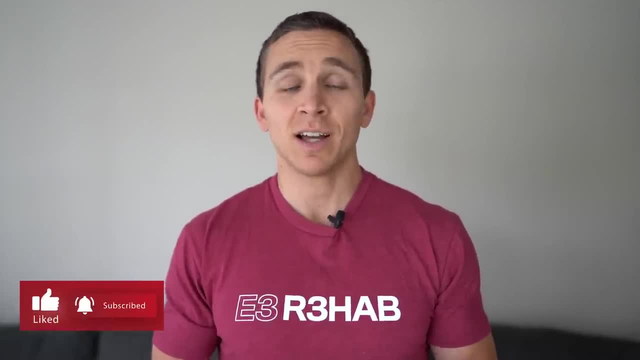 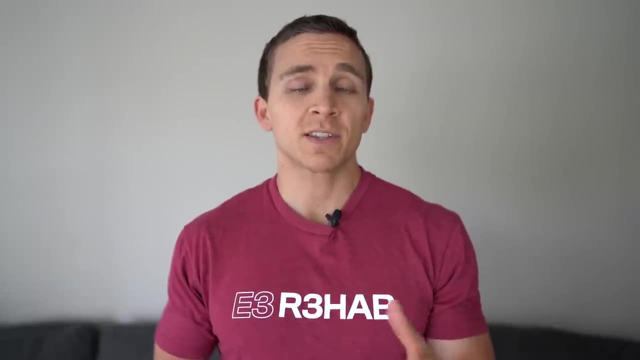 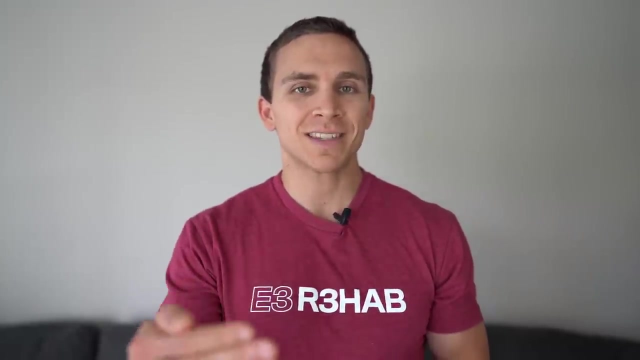 For a sensitive nerve, more isn't always better. So, unlike a lot of exercise recommendations, the goal here isn't instantaneous relief. It's a long-term plan. The movements should be tolerable and shouldn't cause an exacerbation of symptoms later on or the next day. If they do, you probably just need to scale back a bit. 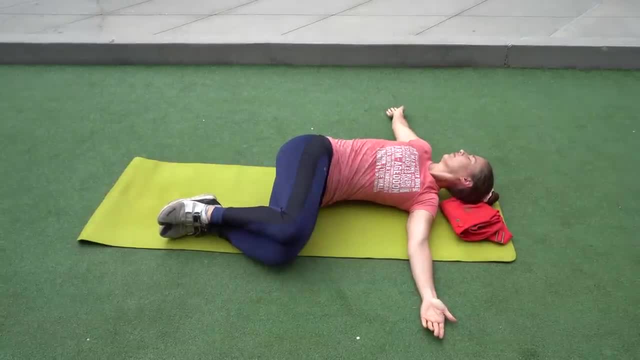 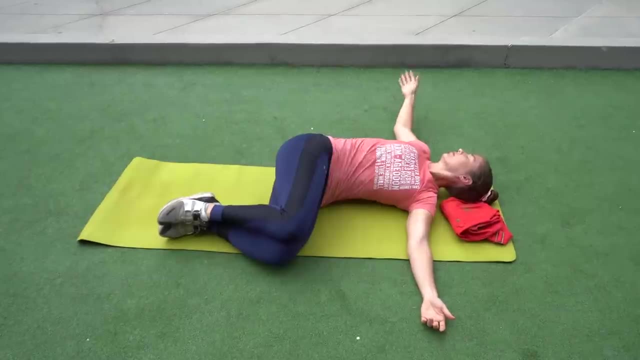 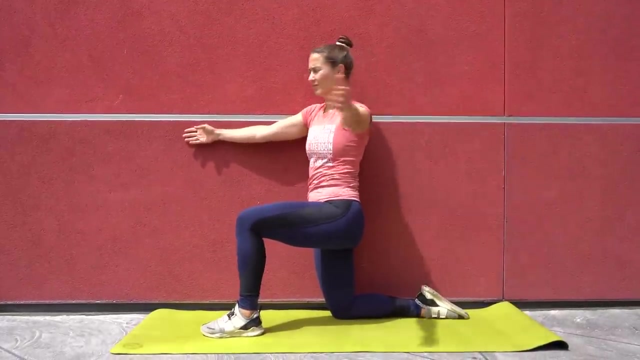 The first exercise is this sideline thoracic rotation, which will guide your cervical spine through rotation and your thoracic spine through extension and rotation, while also moving your shoulder and nervous tissue through a large range of motion To progress this. you can start by stretching your groin back and trying to pick up the next movement and half kneeling.